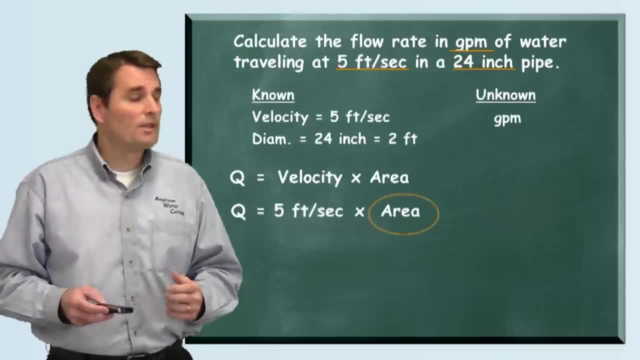 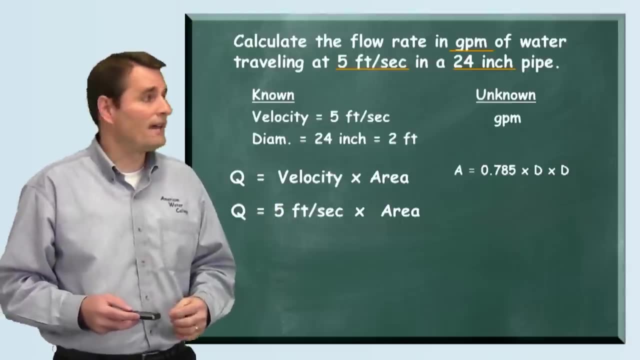 but they didn't give us the area, So we have to calculate that area. Well, to calculate the area of this pipe we use the formula that says: area equals 0.785 times the area, times the diameter, times the diameter. So when we plug the numbers in we see that the 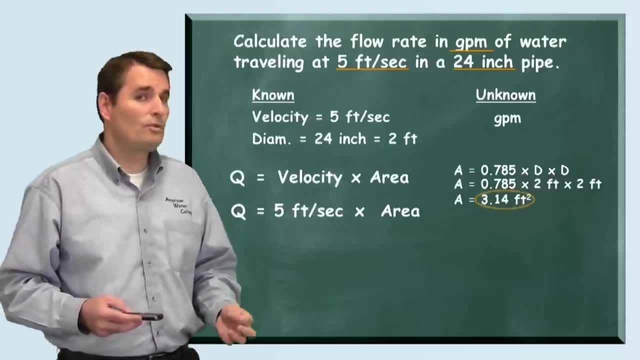 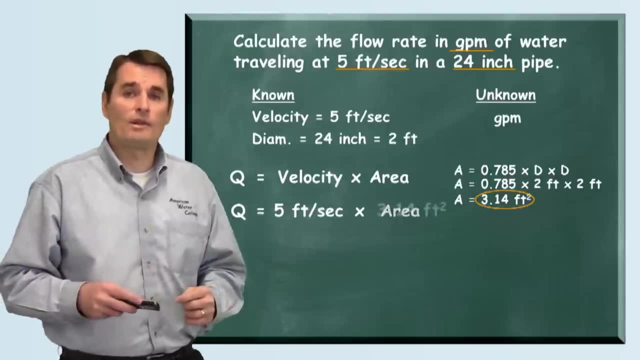 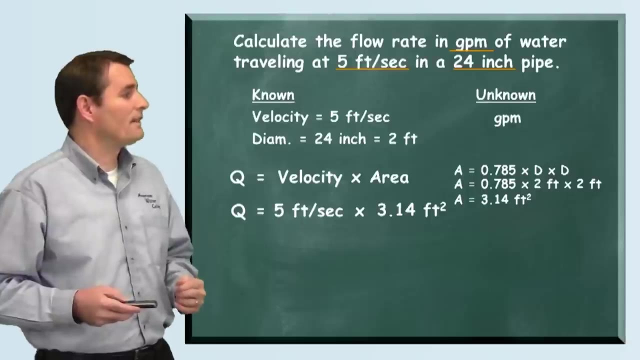 area is equal to 0.785 times 2 times 2, which is 3.14 square feet. Well, now we can plug that square feet into our formula and solve this problem. So when we plug that in, we see that our velocity is 5 feet per second times 3.14 square feet. And when we plug that 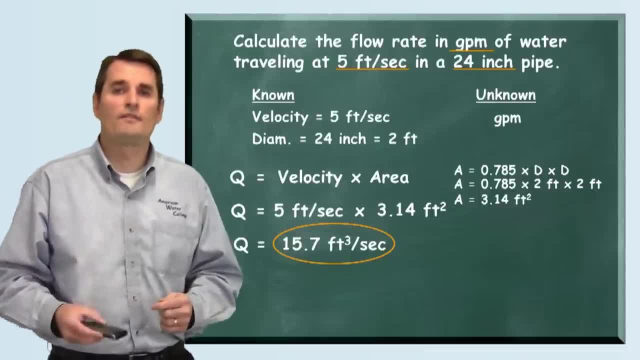 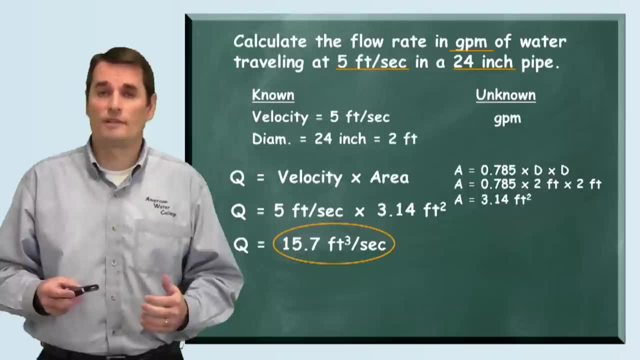 in and when we solve this, we get 15.7 cubic feet per second. So that's our flow rate. However, when we look up under our unknown, we see that the units required for this problem are gallons per minute. Well, we just solved for cubic feet per second, So what we'll do? 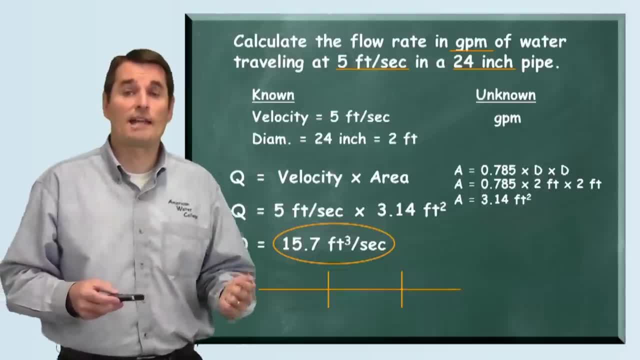 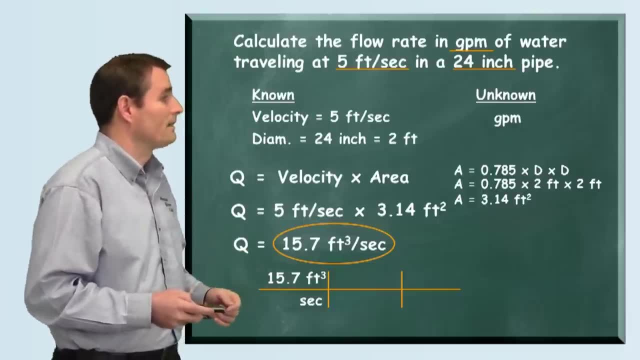 is, we'll do a quick unit conversion to get cubic feet per second to gallons per minute, And here's how that'll look. We'll start with our 15.7 cubic feet per second and we'll go about converting that to gallons per minute. 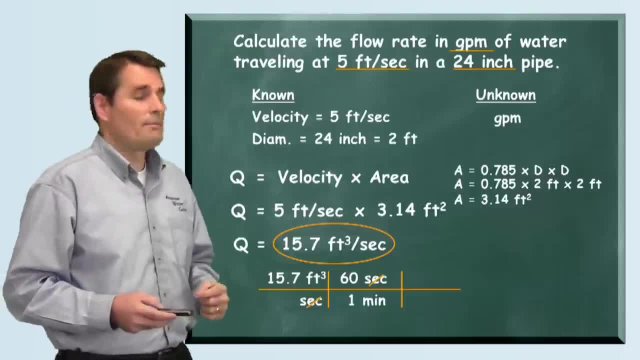 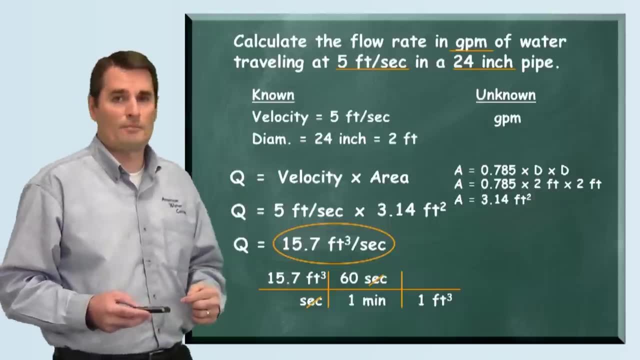 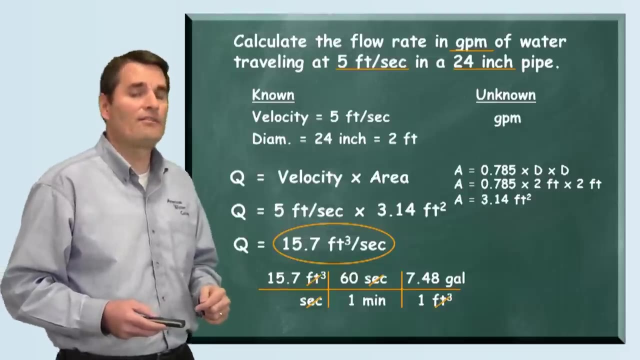 Well, we know that 60 seconds are in one minute, So the seconds cancel out and now we have cubic feet per minute, But we need gallons per minute. Well, there's a conversion that goes between cubic feet and gallons and that says one cubic foot is 7.48 gallons, So the 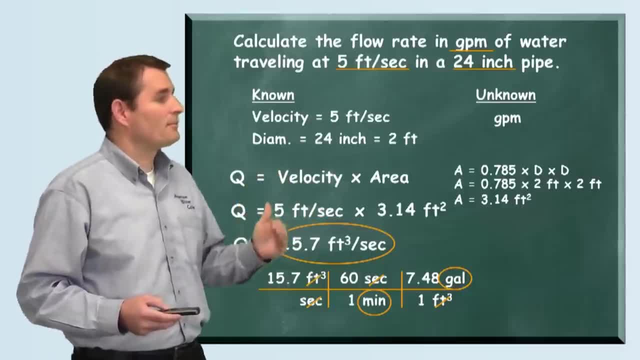 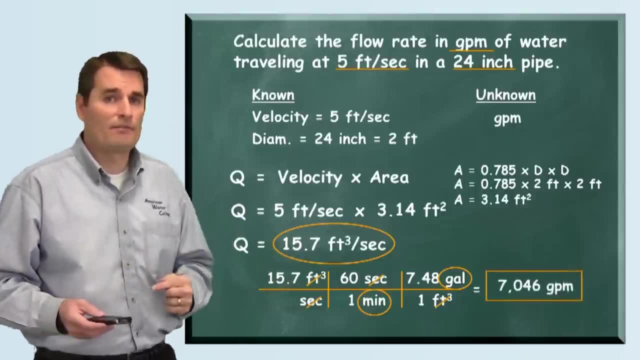 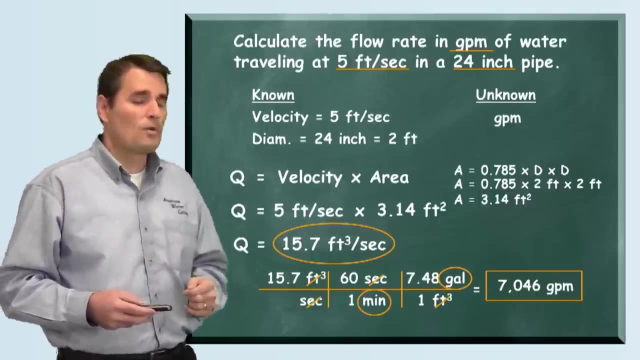 cubic feet cancel each other out, We're left with gallons per minute, which is what we want. So now we simply do the math. You multiply across on the top and divide by the number on the bottom, And when we do that, you can see that our answer is 7,046 gallons per minute. And that, my friend, is how that problem is solved.